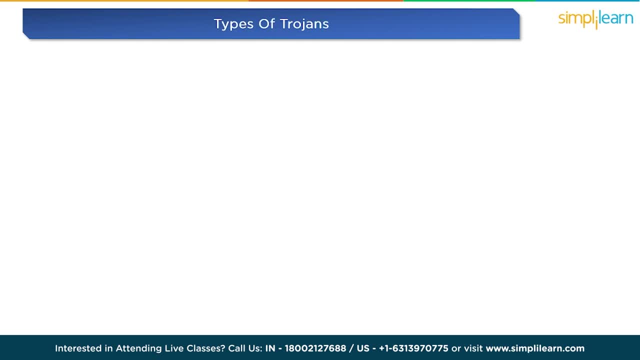 Now that we know the basics, let's look at the different types of Trojans out there. The first one is Remote Access Trojans, or RATS. These sneaky Trojans allow hackers to gain unauthorized access to a victim's computer remotely. They can spy on users. 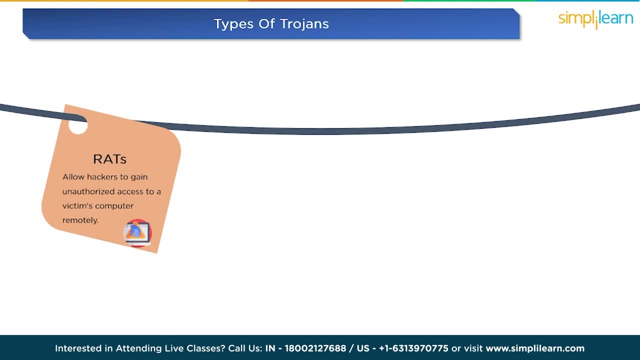 steal sensitive data and even control the infected system. Key Loggers- Trojans- silently record keystrokes, capturing sensitive information like passwords, credit card numbers and other personal data. They can be incredibly dangerous, especially if you use online banking or make online purchases. 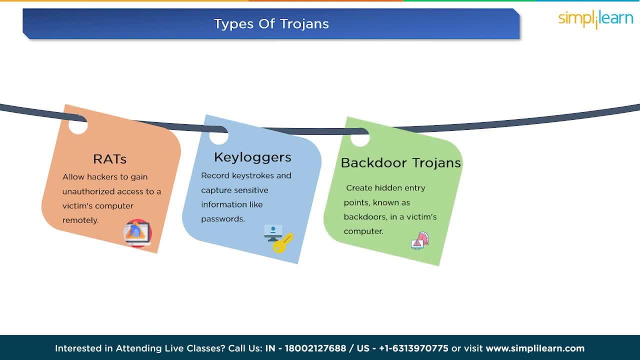 Backdoor Trojans. Backdoor Trojans create hidden entry points, known as backdoors, in a victim's computer. Once installed, they grant cybercriminals full control over the infected system, Eventually leaving it wide open for further attacks. The last one is Downloaders. Downloaders, as the name suggests. download. 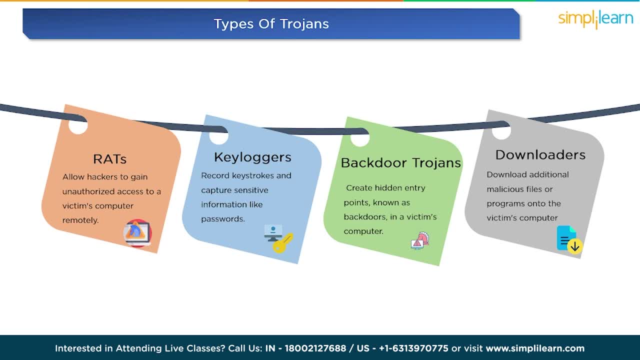 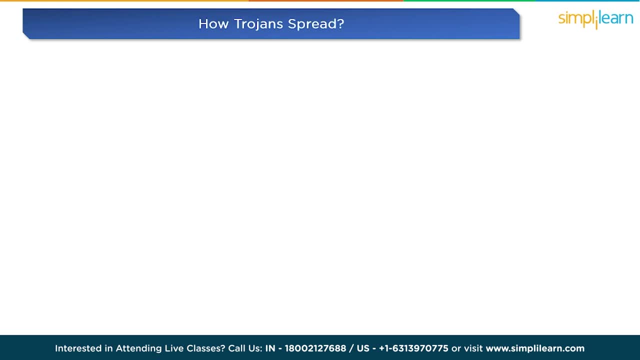 additional malicious files or programs onto the victim's computer. They are often used to deliver more harmful malware to the system. You might be wondering how the Trojan spreads in first place, So let's shed some light on that. The first is Phishing Emails. Phishing emails are one of the most common 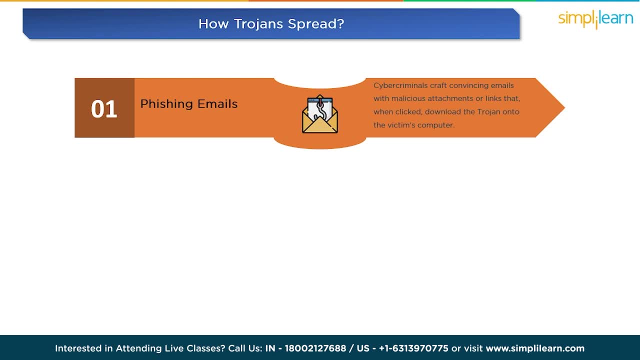 ways Trojans infiltrate systems. Cybercriminals craft convincing emails with malicious attachments or links that, when clicked, download the Trojan onto the victim's computer- Malicious Websites. Visiting compromised or malicious websites can also lead to unintentional Trojan downloads. These sites exploit vulnerabilities in your 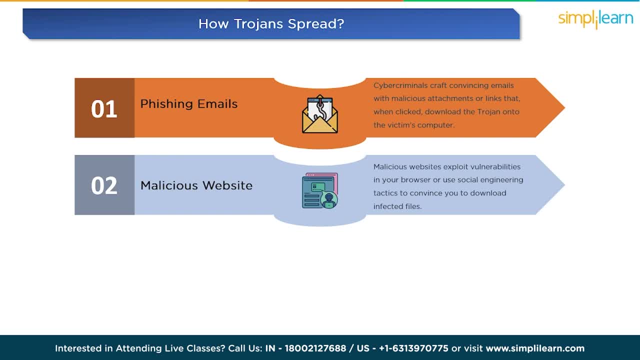 browser or use your social engineering techniques to convince you to download infected files. Software Downloads. Even seemingly legitimate software downloads from untrustworthy sources can be infected with Trojans. Always download software from official and reputable sources. Always download software from official and reputable sources. 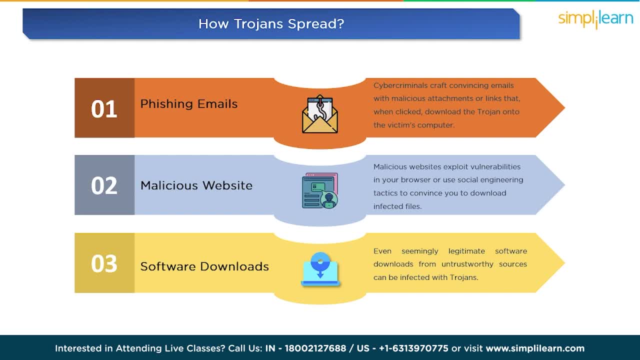 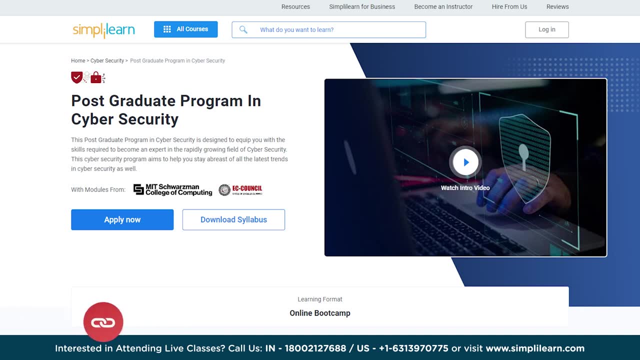 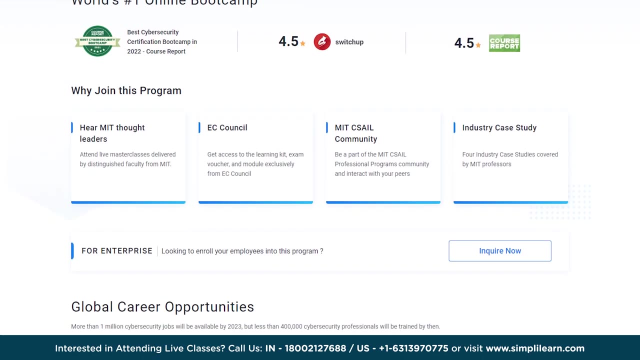 Also, if you want to master the field of cybersecurity, then SimplyLearn's postgraduate program in cybersecurity, in collaboration with MIT, is clearly the right choice for you. This postgraduate program in cybersecurity is designed to equip you with the skills required to become an expert in the rapidly growing field of cybersecurity. 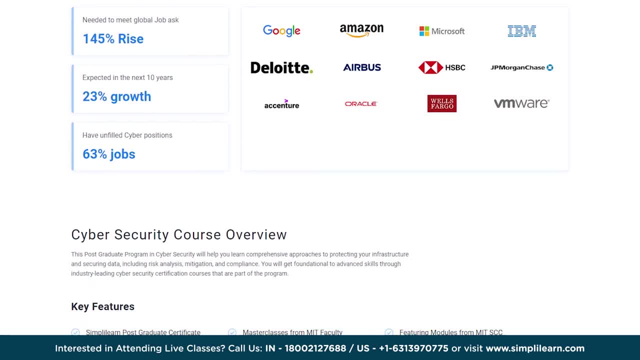 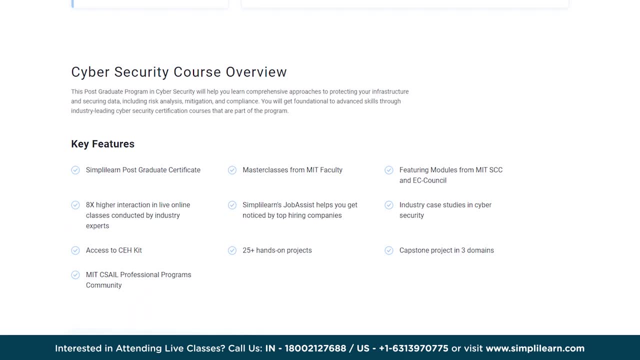 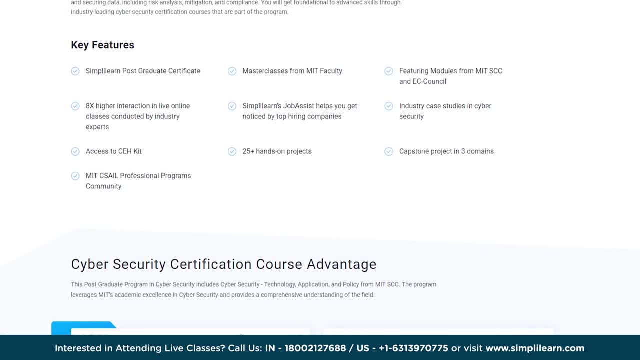 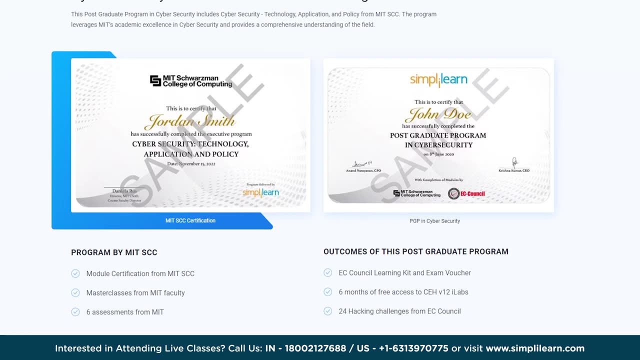 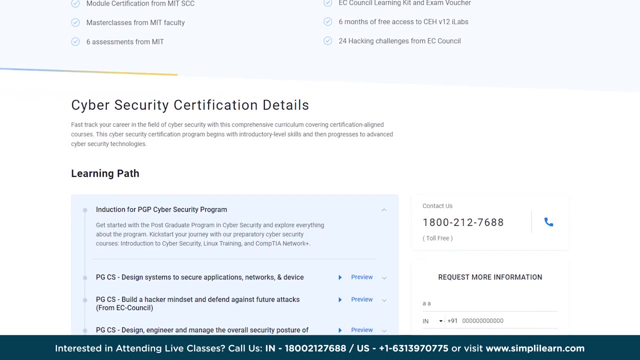 and many more. This cybersecurity certification program begins with introductory level skills and then progresses to advance cybersecurity technologies. This program covers all the essential skills you will need to become an expert in the field of cybersecurity. Cybersecurity is definitely one of the top concerns of businesses today, in any industry. 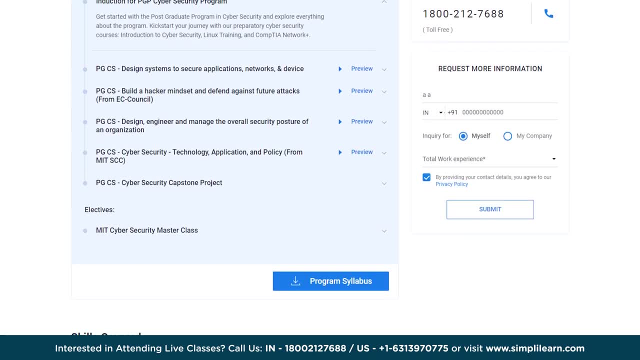 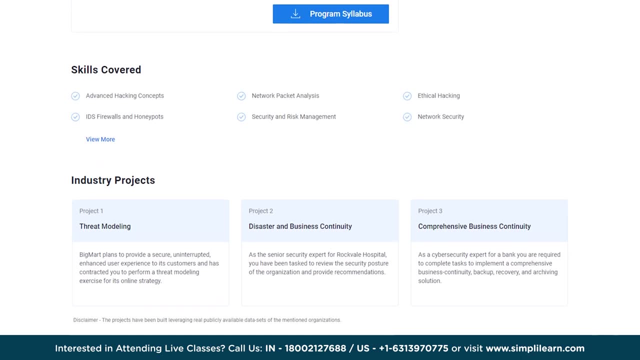 From securing data to anticipating cyberattacks, cybersecurity programs can become a key part of the development of the cybersecurity sector. We are constantly working hard to improve cybersecurity and placing enterprise-wide safeguards to prevent them. employers worldwide are increasingly looking for qualified cybersecurity professionals to join them. 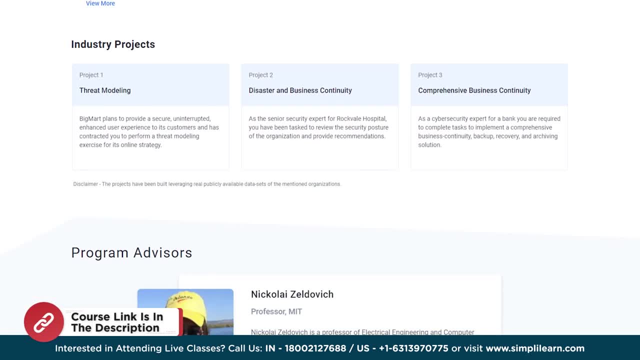 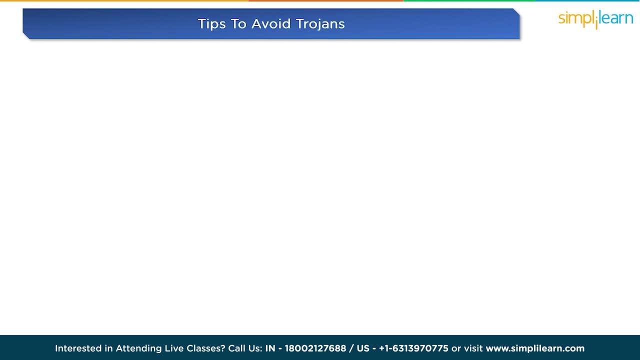 So what are you waiting for? Find the course link mentioned in the description box below and enroll today. Now that we understand the potential risks, let's explore some essential tips to protect ourselves from Trojans. Number one is keep your software updated. 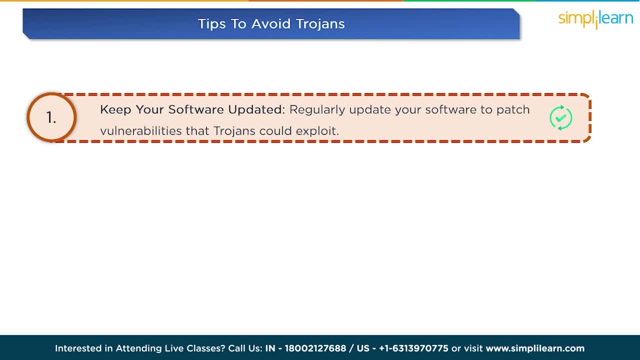 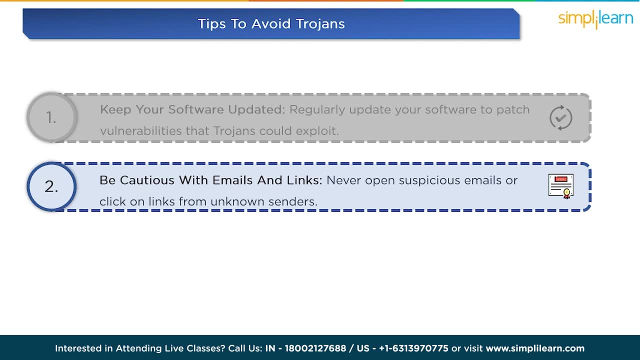 Regularly update your operating system, web browsers and security software to patch vulnerabilities that Trojans can exploit. Be cautious with emails and links. Never open suspicious emails or click on links from unknown senders. Verify the sender's identity before opening any attachment. 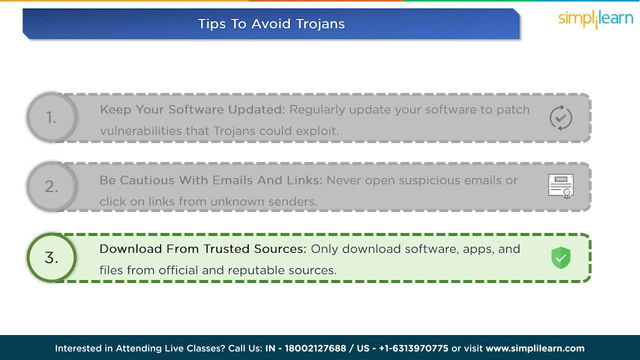 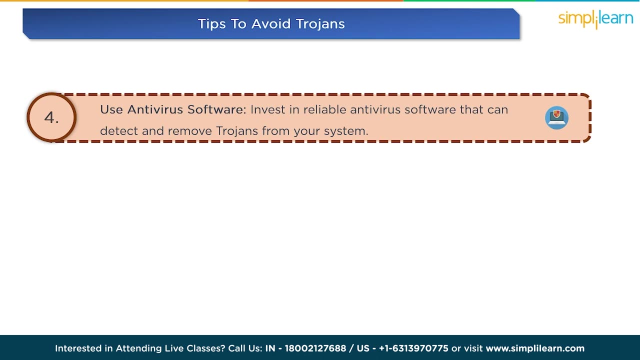 Third is download from trusted sources. Only download software, apps and files from official and reputable sources. Avoid shady websites and torrents. The fourth is use antivirus software. Invest in reliable antivirus software that can detect and remove Trojans from your system. 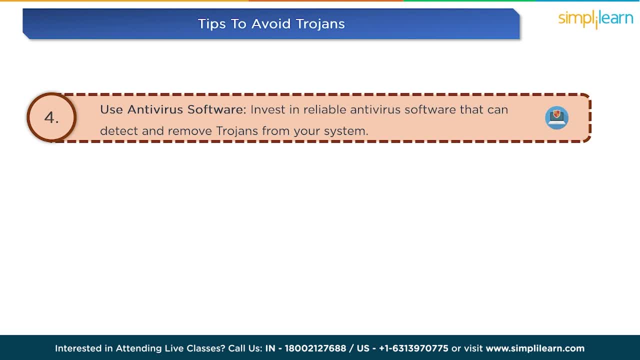 In conclusion, Trojans are dangerous and deceitful cyberthreats that can cause severe damage to your computer and compromise your personal information. However, armed with knowledge and proper security measures, you can protect yourself from falling victim to these malicious attacks. A lot of individuals have attained high salaries and better career opportunities through our 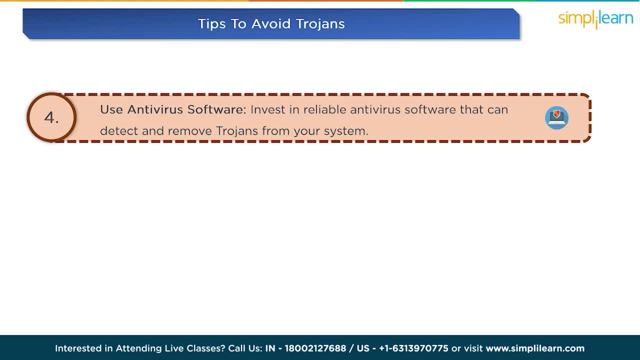 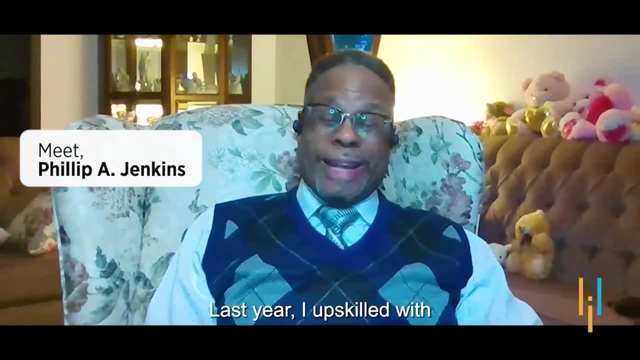 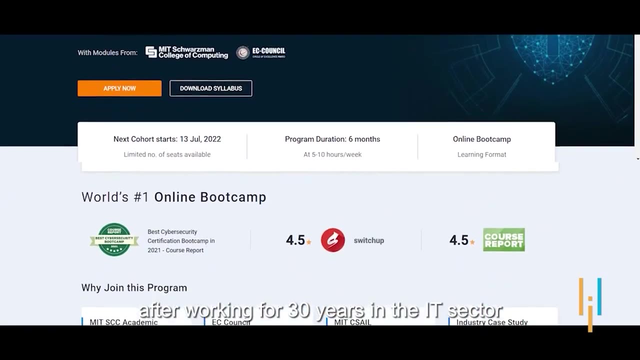 postgraduate program in cybersecurity in collaboration with MIT University. So let's take a minute to hear it out. Hi, I'm Phillip, I'm 61 years old and last year I upskilled with Simply Learn's postgraduate program in cybersecurity, after working 30 years in the IT sector in various different profiles. 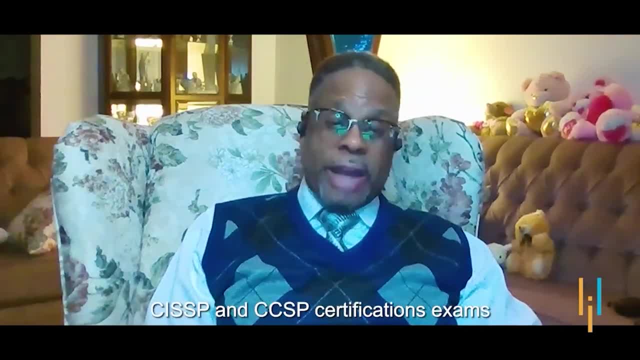 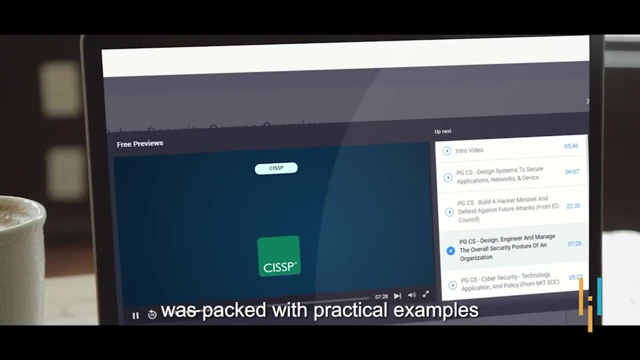 I'm happy to tell you that I was able to clear and pass my CISSP and CCSP certification exams on the first attempt after taking the course. The course, I must say, was packed with practical examples and was led by highly skilled and 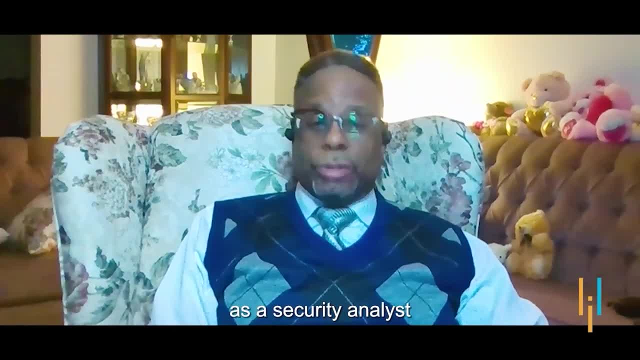 certified instructors. I worked with many companies before as a security analyst in the R&D department. I worked with many companies before as a security analyst in the R&D department. I worked with many companies before as a security analyst in the R&D department.